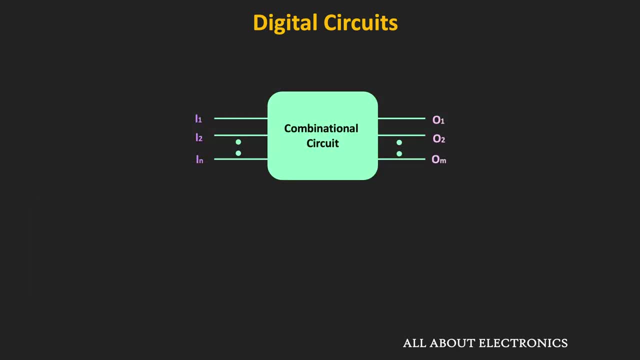 So in the conventional circuit, if you see, then for a given set of inputs, every time we used to get the same output. But in the sequential circuits, for a given set of inputs, we may not get the same output, Because in the sequential circuits the output also depends on the present state of the memory. 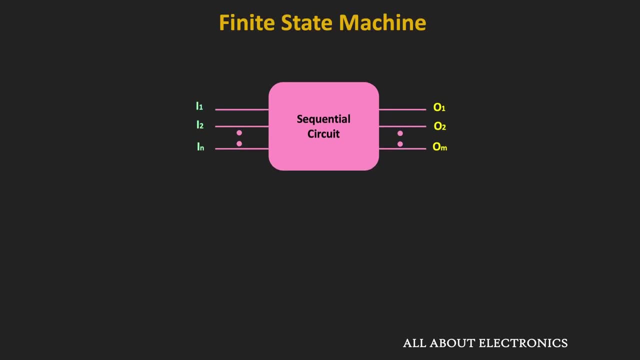 elements. So all the synchronous sequential circuits are known as the finite state machine, Or, in other words, this finite state machine is an abstract model for describing the sequential circuits. So all the synchronous sequential circuits which we have discussed earlier, like the synchronous counters or the registers, are the example of the FSM. 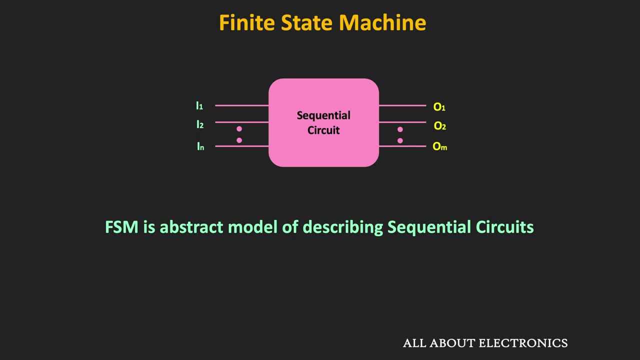 And the reason it is known as the finite state machine is because it has finite numbers. So each FSM has a set of inputs and outputs and a finite set of internal states. Now in this finite state machine, depending on how the output is generated, we have two. 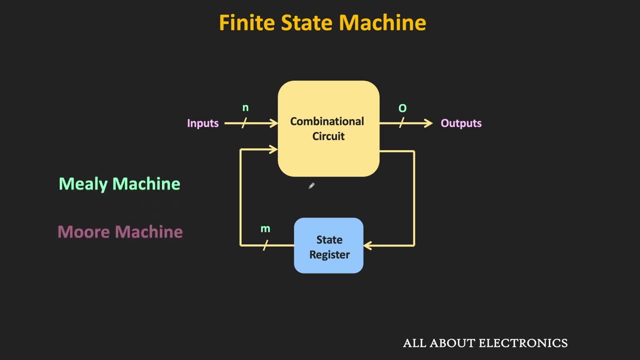 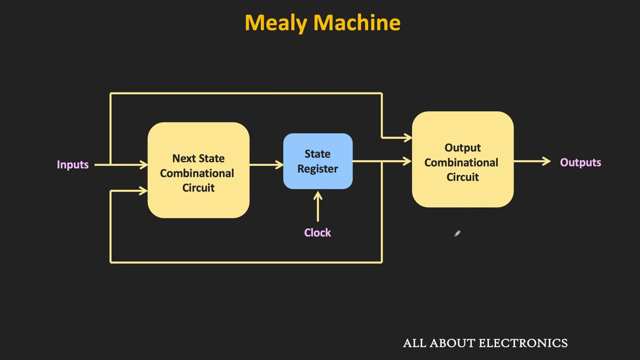 FSM models, That is, the Millie machine and the Moore machine. So in the Millie machine the output is a function of the present inputs as well as the present state of the internal memory elements. So, as you can see, in the Millie machine, first this conventional block. 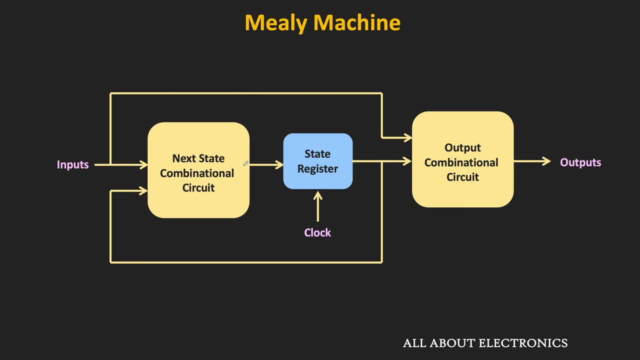 Generates the input for the memory element And, according to those inputs, at the next clock age the state of the memory element will change. So, basically, this conventional logic will decide the next state of the memory element. So, as you can see, the input to this conventional block is the external inputs as well as the 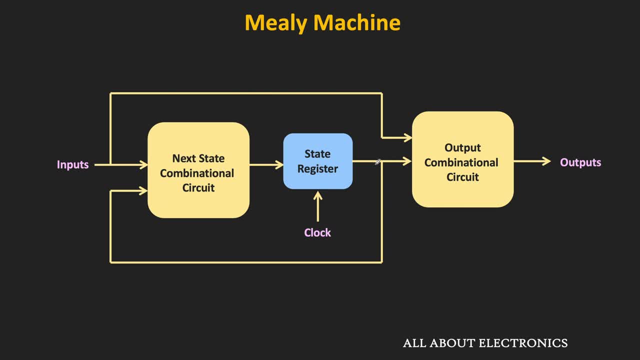 present state of the memory element And the present output of this memory element is going to the output conventional circuit. So this output conventional block will generate the output of the overall circuit. Now, in case of the Mealy type finite state machines, the present external inputs will: 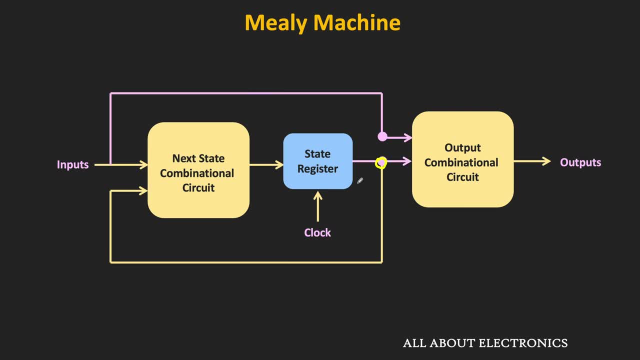 also be the inputs to this output conventional block. So if we see the overall output of the Mealy machine, then it is the function of the present state of the memory element as well as the present inputs to the circuit. On the other hand, in the Moore machine, the only difference is that these external inputs 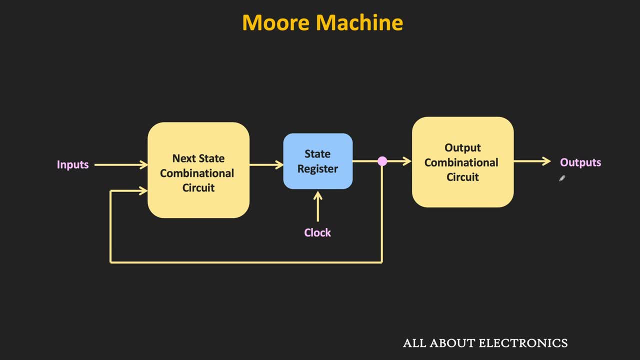 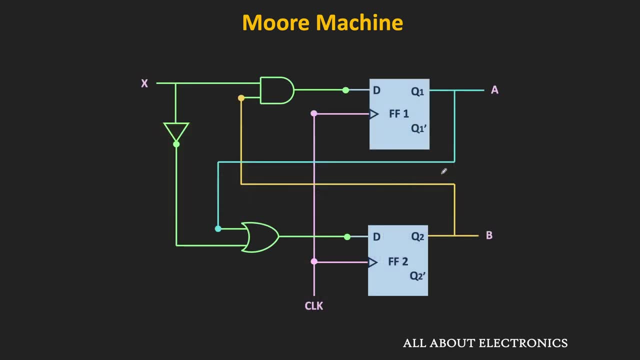 are not connected to this output block. That means in the Moore type finite state machine the output is the function of only the present states of the memory element. So if you see this sequential circuit then it is the example of the Moore machine. 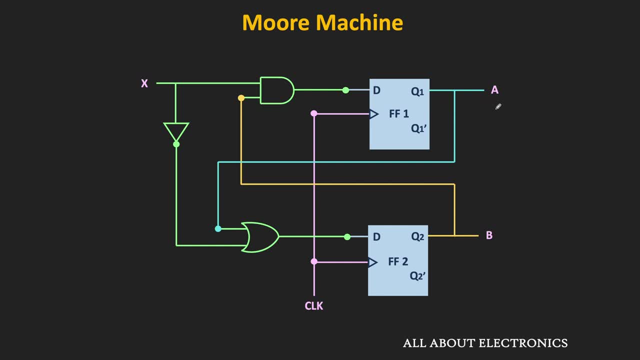 Because in this case, if you see, then this output, A and B, depends on the output of these two flip-flops. So if you see over here, then this logic gates generates the input for these two flip-flops. So basically it is a next state combinational block. 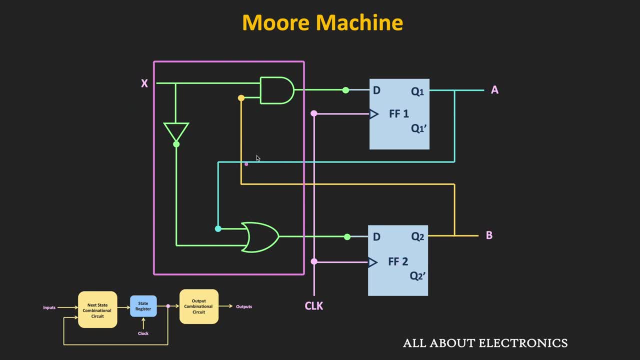 So here, based on this input, This logic gates will generate the two inputs for these D flip-flops, And based on these two inputs, the next state of the flip-flops will get decided, And the output of these two flip-flops represents the present state of the memory element. 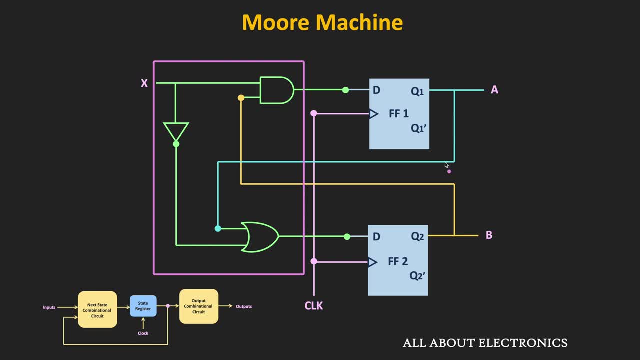 So, as you can see over here, the output of these two flip-flops is going back to the logic circuit. That means the input to this combinational block is the external input x as well as the present state of the memory element, And in this case 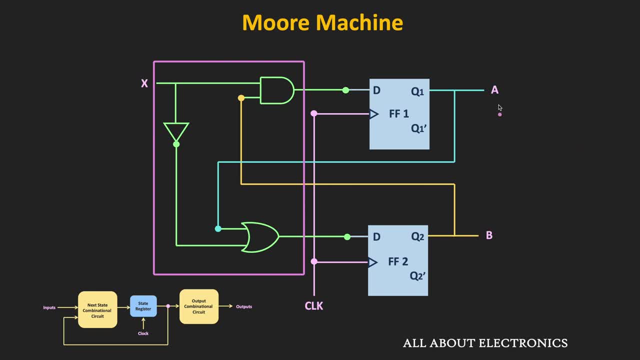 We do not have any output. combinational block. That means here the output of these two flip-flops represents the output of the circuit, But typically we can also have the combinational logic at the output side, which will generate the final output. 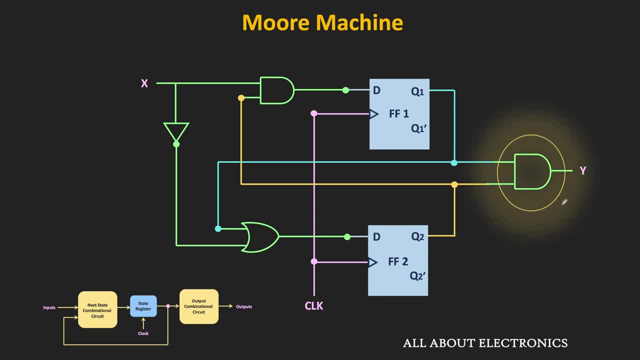 So, for example, in this case we have this AND gate at the output side And, as you can see, the output of these two flip-flops are connected to this AND gate. That means here the output of this AND gate will represent the output of the overall circuit. 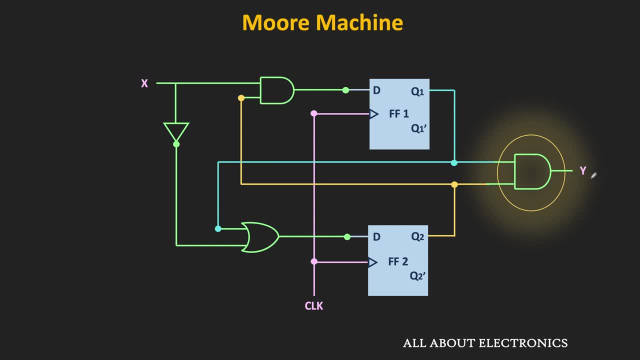 So in this case, as you can see, the output of the circuit depends only on the present state of the flip-flops, And that is why this circuit is an example of the Moore machine. On the other hand, in the Millie machines, the external inputs are also connected to. 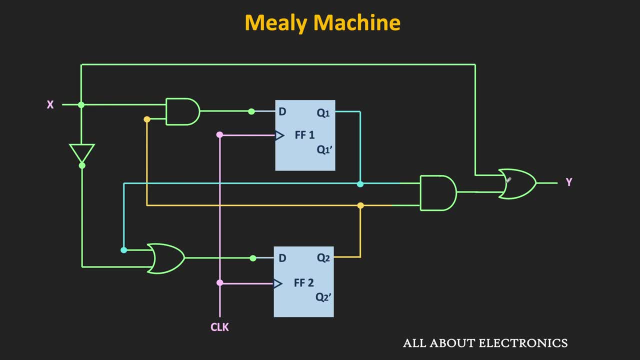 the combinational logic at the output side. So, for example, this sequential circuit is an example of the Millie machine. So this circuit is similar to the earlier circuit, but here this OR gate is connected at the output side. So, as you can see, this input x is one of the inputs to the OR gate, while the second 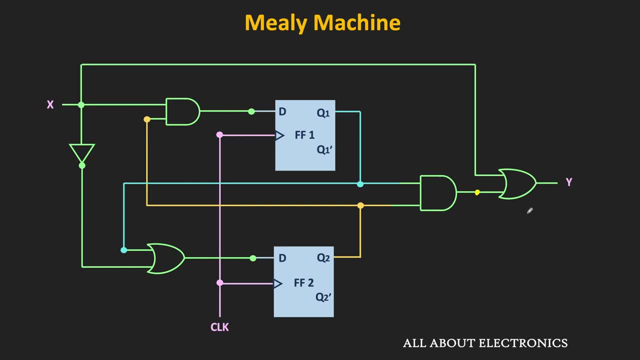 input is the output of this AND gate. So in this circuit, this output y depends on the present input, x as well as the present states of the flip-flop. So, in short, depending on how the output is generated. for the circuit we have two. 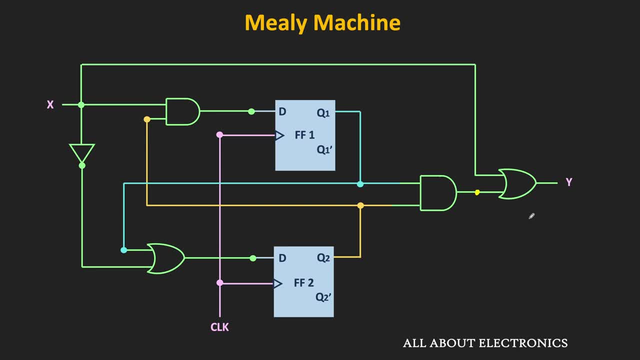 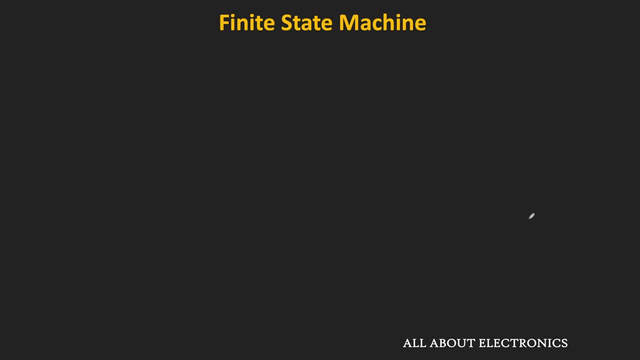 FSM models, that is, Millie machine and the Moore machine. But irrespective of the type of the FSM, the behavior of the machine can be represented in the three different ways. The first one is the State Transition Diagram. So this State Transition Diagram is a pictorial way of representing the behavior of the FSM. 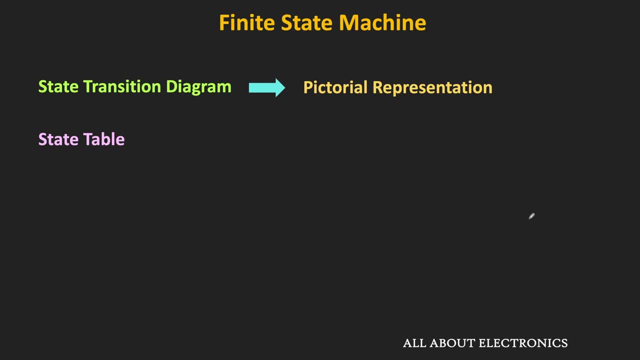 The second one is the State Table, So this State Table represents the same information in a tabular form. And the third one is the State Equations, which is the algebraic way of representing the same information. So, using any one of the three methods, we can describe the behavior of the FSM. 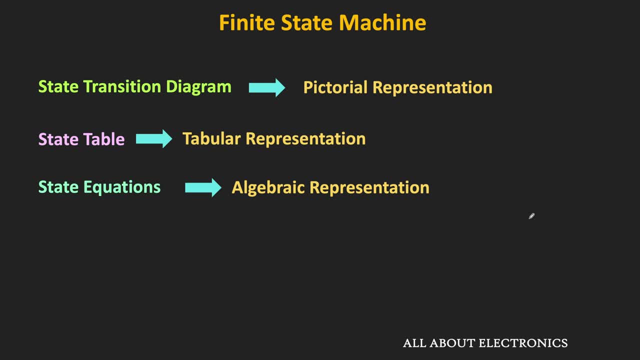 So In the earlier videos of the flip-flop and the counters we have already discussed about the state table and the state equations, But we haven't talked much about the state diagram. So in this video let's understand it in detail. 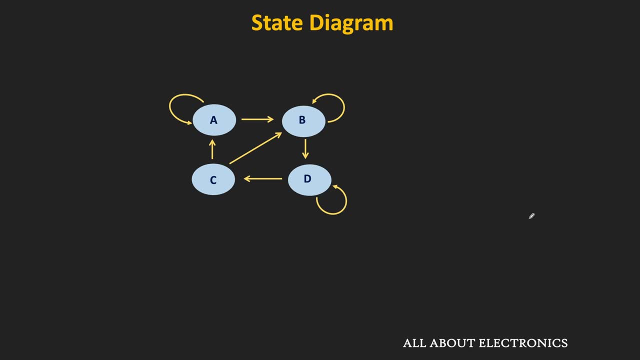 So, like I said, the state diagram is a pictorial way of representing the behavior of any finite state machine or the sequential circuit. So in the state diagram every possible state is represented as a circle. For example, in the given state diagram we have total 4 possible states. 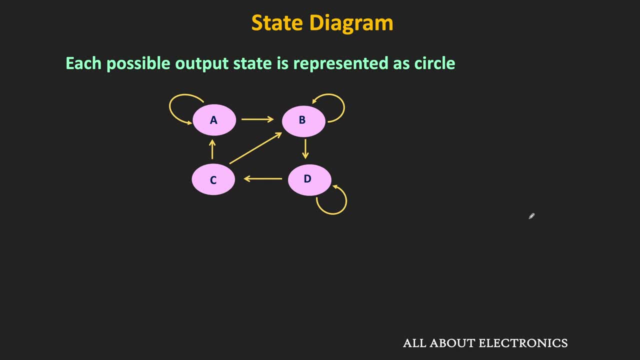 So all the states are represented in the circle And to differentiate all the different states, each state is assigned a specific value. So in this case, as you can see, the each state is represented with a different character, But typically the each state is assigned the binary value. 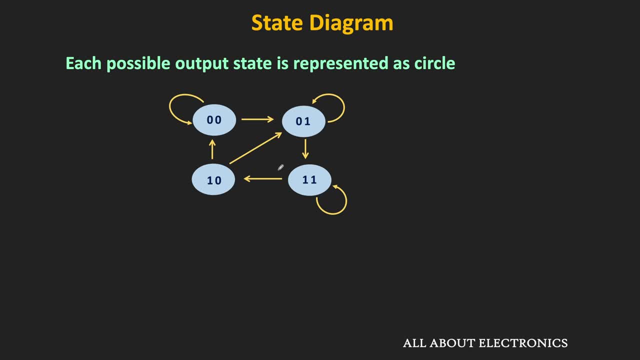 So, as you can see over here, since we have 4 states, so each state is represented with the 2-bit numbers. That means in the state diagram the every possible output state is represented as a circle And in this state diagram the transition from the one state to the other state is represented. 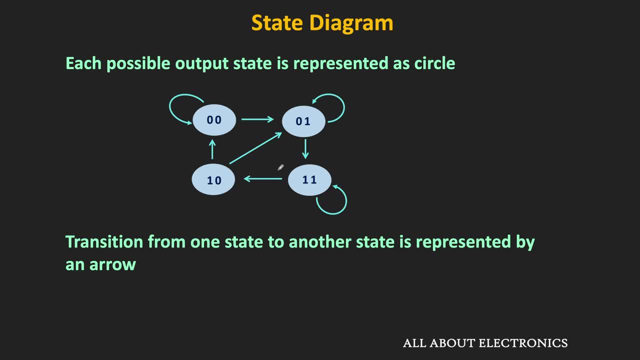 by the arrow. So here these arrows represent the transition from the one state to the other state And the binary value on top of these arrows represents the input value which will lead to this state transition. For example, if the current state of the circuit is 0, 0.. 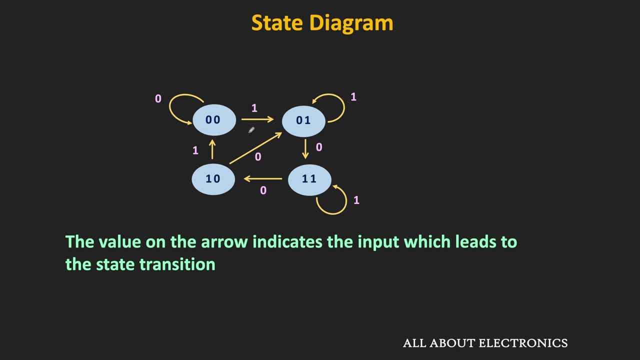 And when we apply the 1, 0. As an input, then the state of the circuit will change from the 0, 0 to 0, 1.. But in the same state- suppose we apply the 0 as an input- then the circuit will remain. 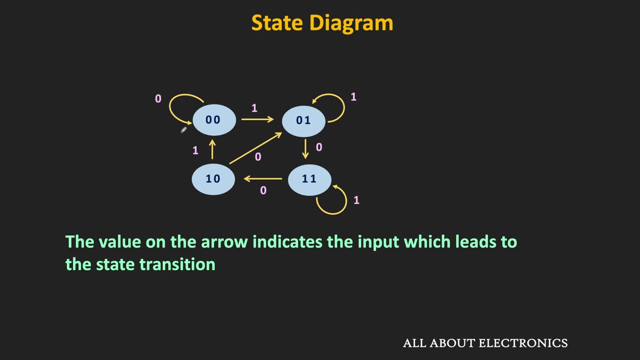 in the same state. So, in this way, the binary value on the top of these arrows represents the input which will lead to this state transition, And the value next to the input represents the output of the circuit corresponding to the specific input. So, for example, if the circuit is in a 0, 0 state, 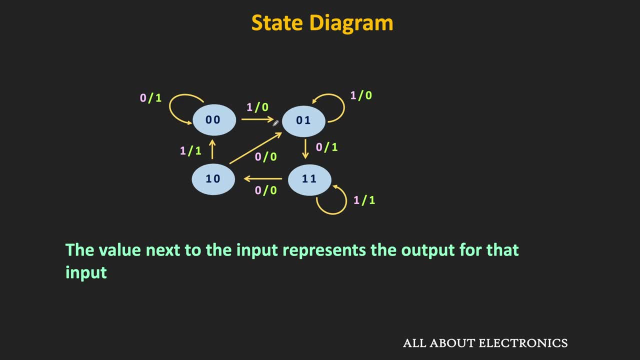 And if we apply the 1 as an input, then, as you can see, the output of the circuit will become 0. And it will go into the 0, 1 state. So that is how this state diagram represents the behavior of the final state machine for 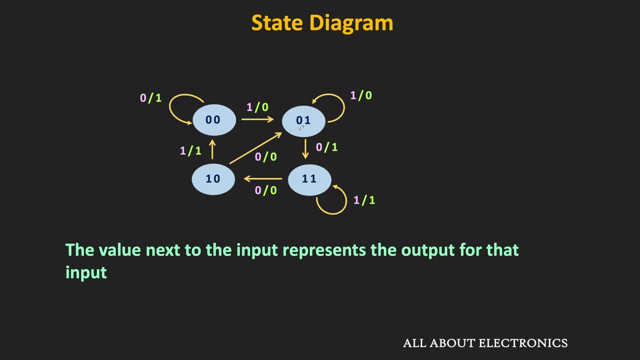 any sequential circuit in a pictorial way. So from the state diagram we can get to know the number of inputs and outputs, as well as the number of states of the final state machine, And it also shows that how the change in the input leads to the state transition and the 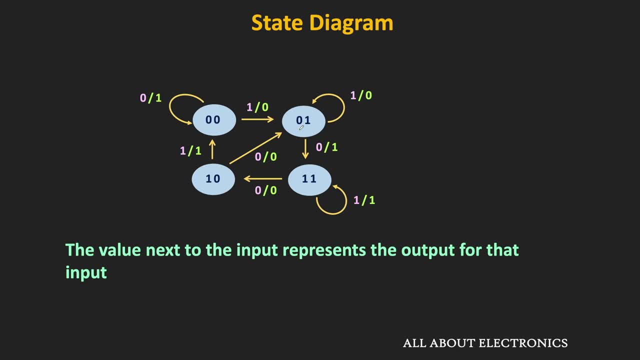 change in the output. So there you go. So this state diagram is a diagram of the Millie machine Because, like I said, in the Millie machines the output is a function of both present states and the input, And that is why over here these outputs in a green color are represented just beside. 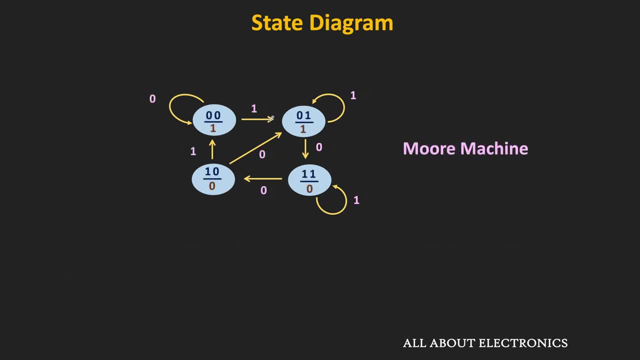 the inputs. But in the Moore machines the output is a function of only the present state of the memory elements, And that is why in the state diagram of the Moore machines the output is represented in the circle itself. For example, in this case this binary value in the brown color inside each circle represents: 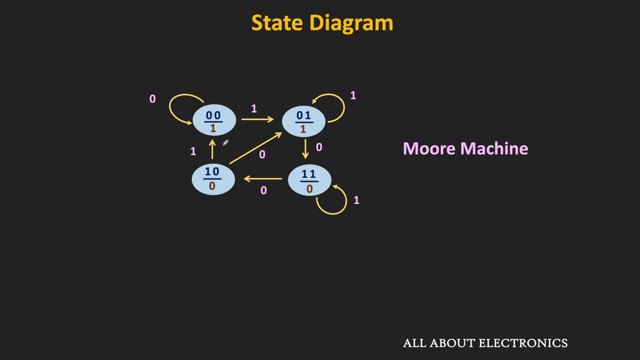 the output of the circuit corresponding to the specific state. So that is the basic difference in the state diagram of the Millie machine and the Moore machine, And from this state diagram we can easily draw the state table. So the state table represents the same information in a tabular form. 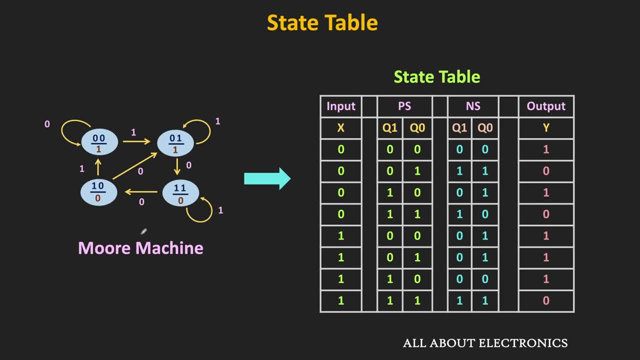 For example, this is the state table corresponding to the given state diagram. So, as you know, the state table consists of the inputs. This state table represents the inputs and outputs of the circuit, as well as the present state and the next state of the sequential circuit. 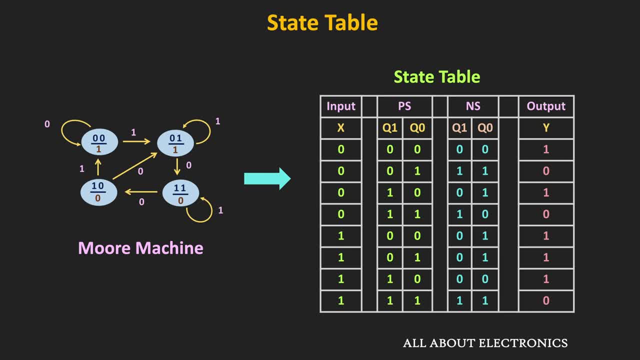 So if you see the state diagram, then here we have 1 input and the 1 output. So let's say the variable for the input is equal to x, while the variable for the output is equal to y, And if you see over here, then we have a total 4 states. 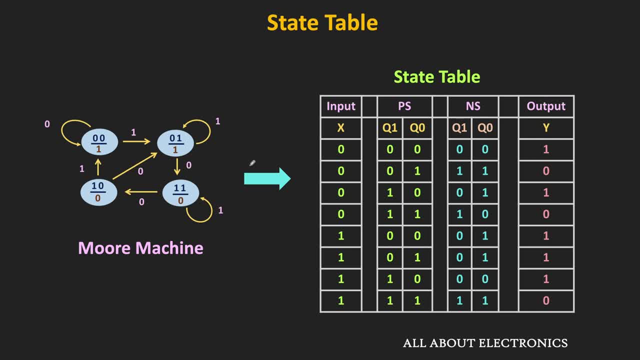 So these 4 states can be represented with the help of the 2 bits. Let's say that is equal to Q1, Q0.. Here, depending on the input and the present state, we will get the corresponding next state and the output. 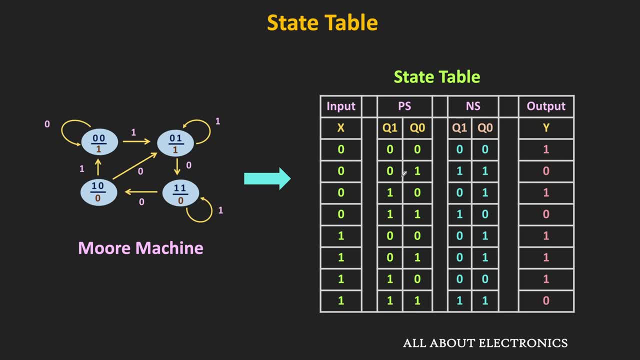 So here for the three variables x, q1, and q0, we have total 8 different possibilities. So here the 8 different possibilities are written, And then from the state diagram we can easily find the next state and the output. 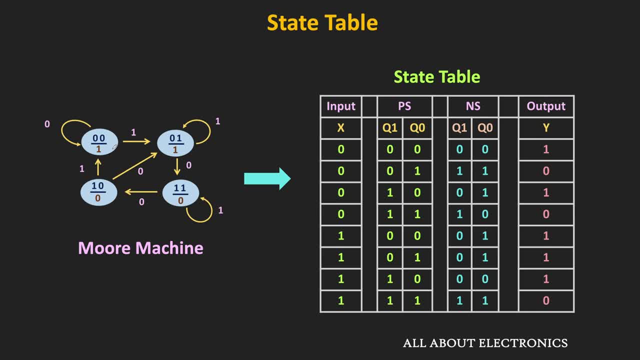 For example, if the circuit is in the state and if the current input is equal to 0,, then the circuit will remain in the same state. That means in that case the next state will be equal to 0, 0.. 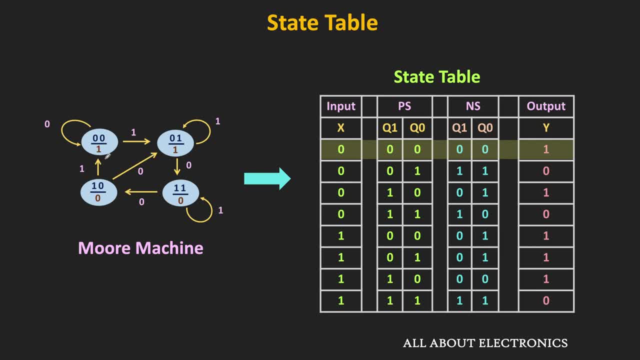 And, as you can see from the state diagram, in the 0, 0 state the output is equal to 1.. That means in this case this y is equal to 1.. Similarly, in the same state, if the input is equal to 1,, then the next state will be: 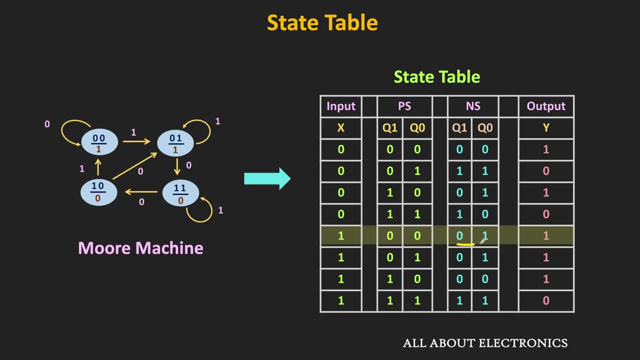 equal to 0, 1.. So in this column we will write 0, 1.. And whenever the output state is equal to 0, 1, then, as you can see, the corresponding output is equal to 1.. 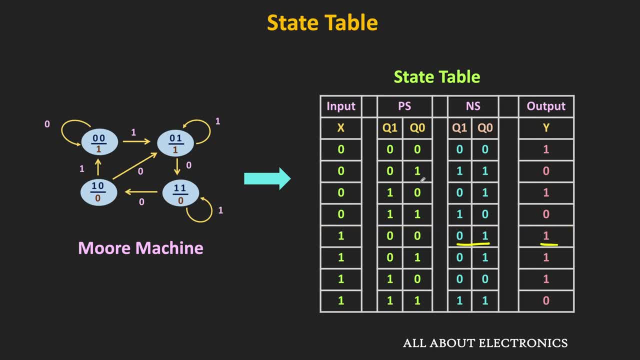 That means here we have the output state, We will write 1. And likewise we can complete the entire table. So in this way from the state diagram we can easily draw the state table. So here this state diagram was for the Moore machine. 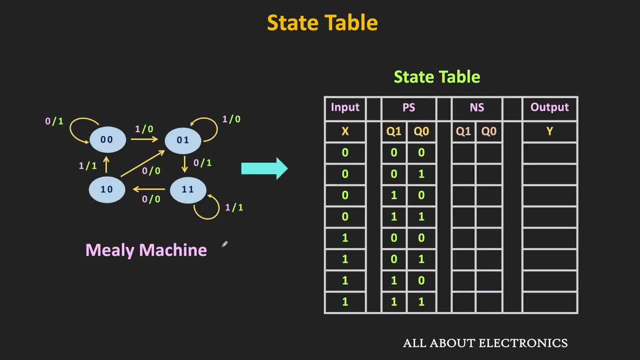 But similarly we can also draw the state table for the Millie machine. So here, as you can see, this is the state diagram of the Millie machine And in a similar fashion we can also draw a state table for this given diagram. 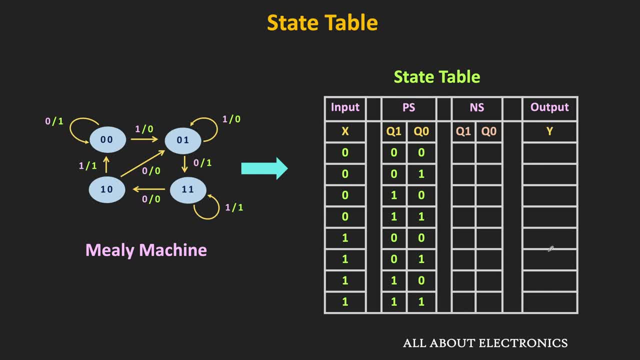 So once again, if you see, Then here we have a 1 input and the 1 output. Let's say the input is equal to x, while the output is equal to y And, as you can see from the diagram, once again we have 4 states. 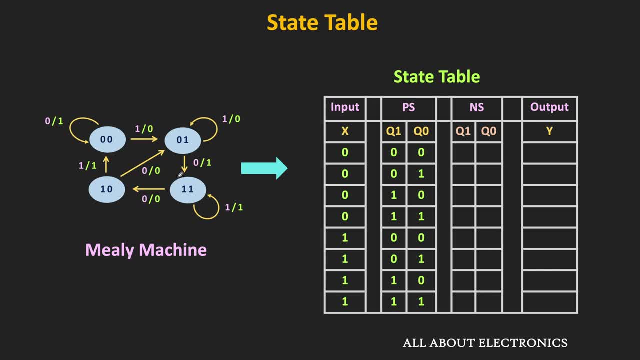 That means these 4 states can be represented with the help of the 2 bits. So once again let's say that is equal to q1, q0.. So here, for the input x and the present state, q1 and q0, we have total 8 different possibilities. 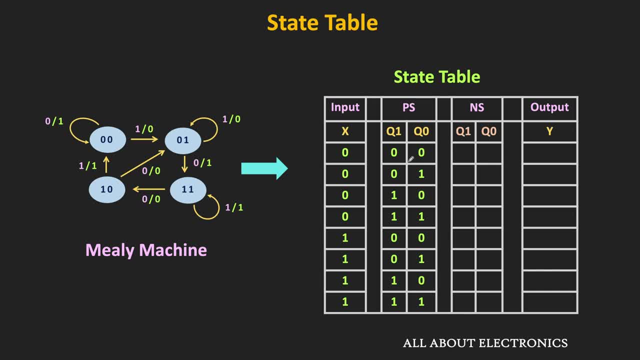 And from the state diagram We can easily find the next state And the corresponding output. So once again, if you see over here, Then for the state 00, when the input is equal to 0, then the circuit will remain in the 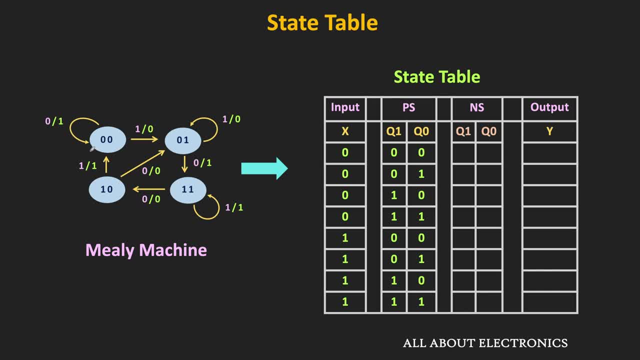 same state. That means if we see the next state, then that will be equal to 00. And in that case this output is equal to 1.. That means in this column we will write 1.. Similarly, currently, if the circuit is in the 01 state and the input is equal to 1,. 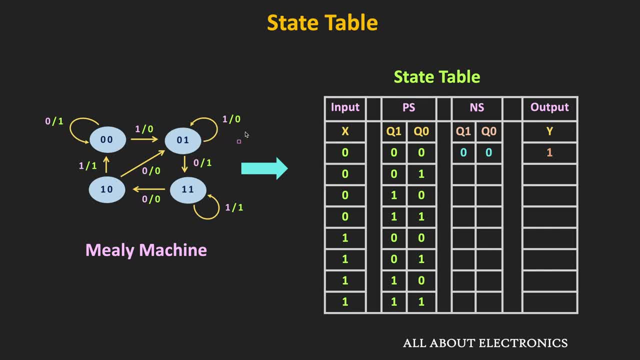 then the circuit will remain in the same state And in that case Its output will remain 0.. So basically, here we are talking about this condition. So in this way, from the state diagram we can easily write the state table. 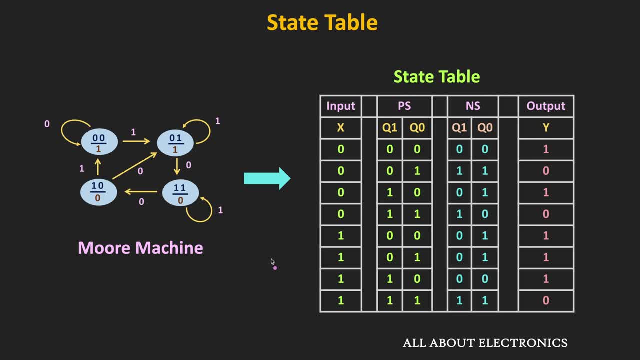 Now if you see the Moore Machines, then in the Moore Machines the output y only depends on the present states of the memory element. That means as the state of the circuit changes, then the output of the circuit will also change. So in a way in a Moore machines this output is synchronized with the clock signals. 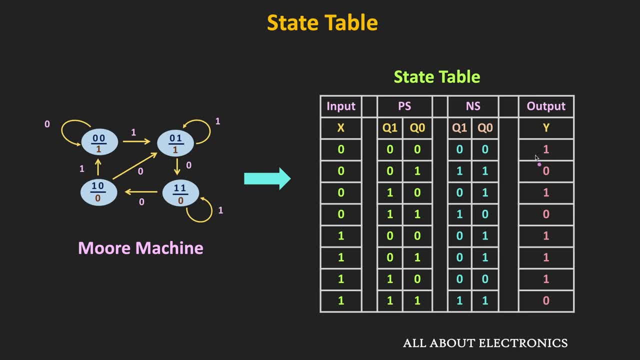 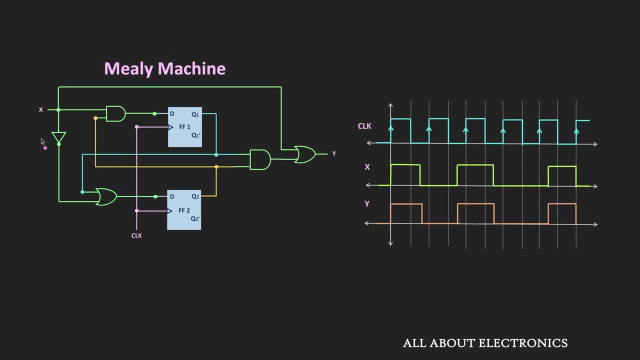 In a way, in a Moore Machines, this output is synchronized with the clock signals, Because at every age of the clock signal the state of the circuit will change, And with the change in the state the output of the circuit will also change. 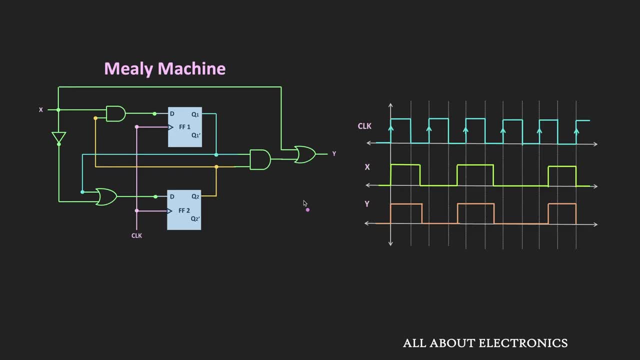 But in the milli machines, as you know, the output of the circuit also depends on the present inputs, That means during the clock cycle. if the input of the circuit changes, then the output of the circuit will also change. For example, for the given milli machine, if the present state is equal to 0,0,, then 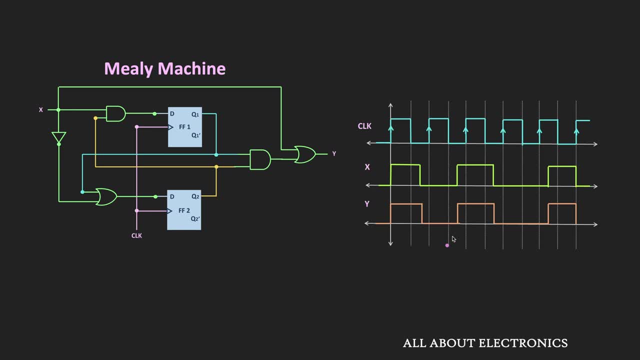 with the change in the input. this is how the output of the circuit will change. So, as you can see, during the clock cycle, if the input changes, then the output of the circuit will also change. So in a way in the milli machines we also need to synchronize the input with the clock.